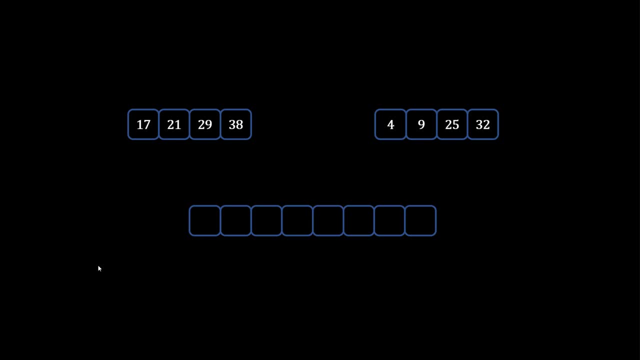 For now. just think you have two sorted array. you want to create one single sorted array out of it. How can you do that? Just pause this video and think about it. It's actually quite simple. So you start with the first element in each of this array. You compare them: The smaller one is 4.. 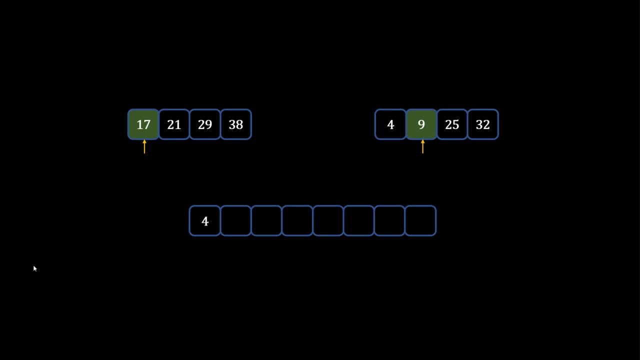 So you put that smaller element into your sorted array. Then you keep the pointer at 7 as is, And in the second array, which is on the right hand side, you have moved your pointer to next element, which is 9.. Now you compare 9 with 17.. Which one is smaller? Well, 9.. So you put 9 here. 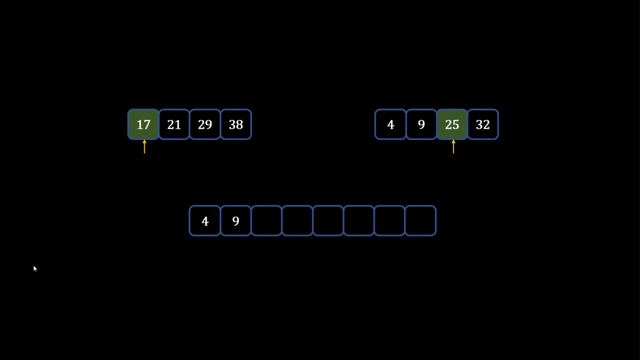 And after you put that into sorted array, you move the pointer. So now you are at 25.. Now you compare 17 with 25.. Which one is smaller? Well, 17.. You put 17 here, And now you move the pointer on the left array. So now you are at 21.. You again compare 21 and 25.. Put 21 here. 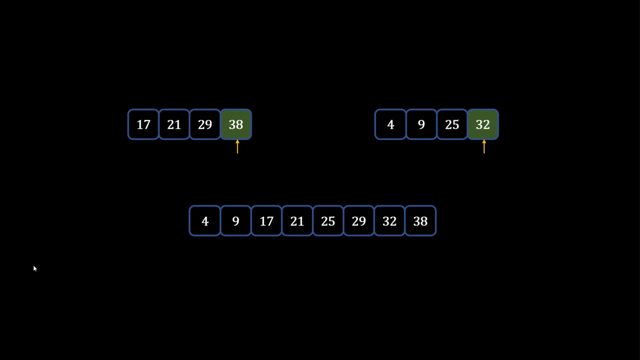 You keep on doing that and you get this nicely sorted array. So what we learned is, if we have two sorted arrays, creating a single sorted array out of it is very easy. So now let's go back to our original problem, which is we have totally random unsorted array. 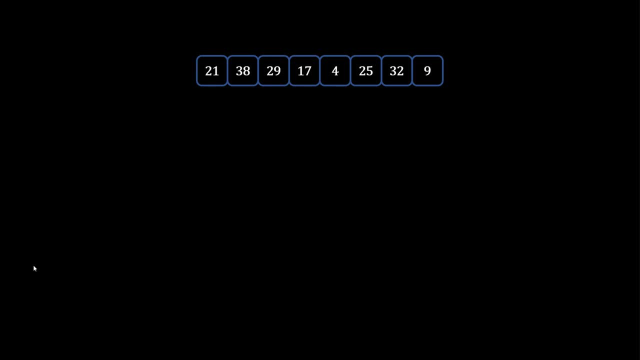 How can you short this using the concept that we just learned? Okay, let's try this out. okay, just for an experiment. We divide this into two arrays, So we take first four elements, next four elements, make it half and half. If you have nine elements, you 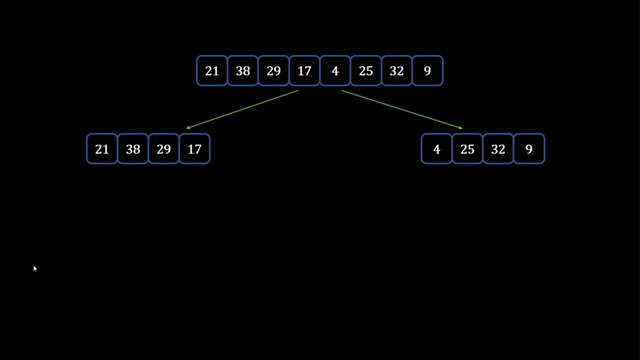 can do four and five, doesn't matter. Then now you have two arrays and you try to merge them. But well, I cannot merge them easily using the techniques I just learned, because these two arrays are not sorted. Hmm, So then what if I try to divide them again? 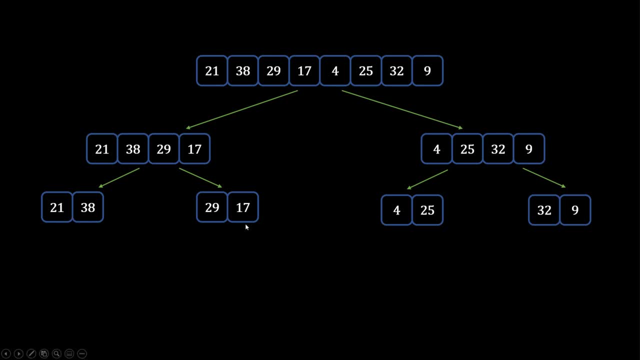 Now can I merge this 21-38 with 29-17?? I still cannot, because these two arrays are also still not sorted. 21-38 is sorted, but 29 and 17 is not sorted. Alright, so then you move to the next step, which is you still divide them. 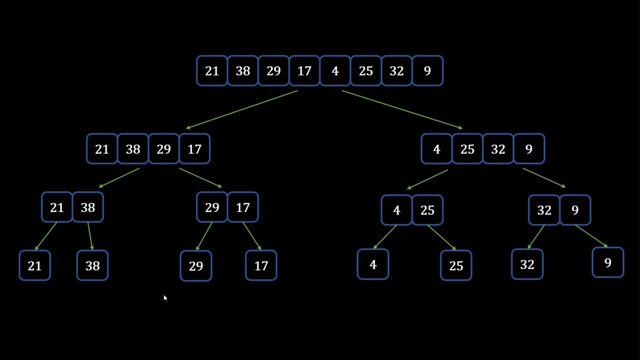 You might have known about divide and conquer and using recursion, and that's exactly what we're doing. we're doing here. now we have all the arrays with only one element. this array has only 21, this has 38, and so on. now can we merge them? well, yes, now we can, because an array with single element is. 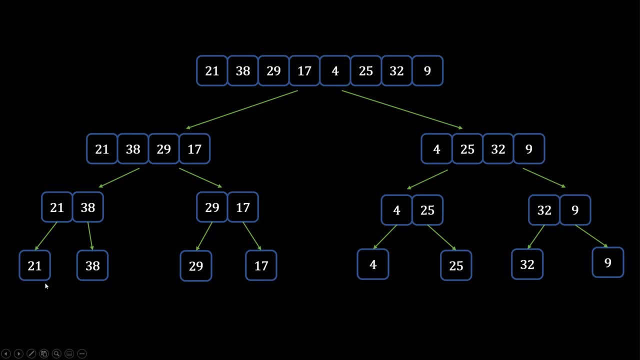 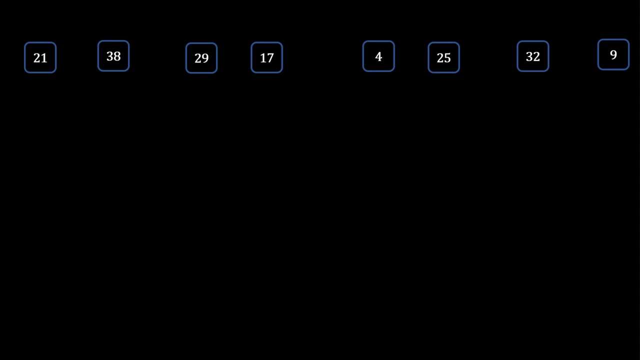 already sorted. so now we can use our technique that we learned initially and merge them. so let's take this eight arrays that we have. although they have single ml element, they are still arrays, arrays with single element. now we go back, take 21 and 38 and try to merge them. well, we can merge. 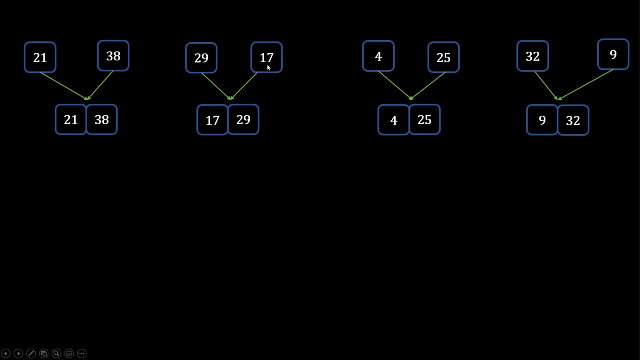 them using the techniques that we learned initially. same thing with 729. it looks like this. 425 looks like this. 932 looks like this. then you go to the next step. so see now you, when you merge these two arrays- 21, 38 and 17, 29, these two are already sorted. 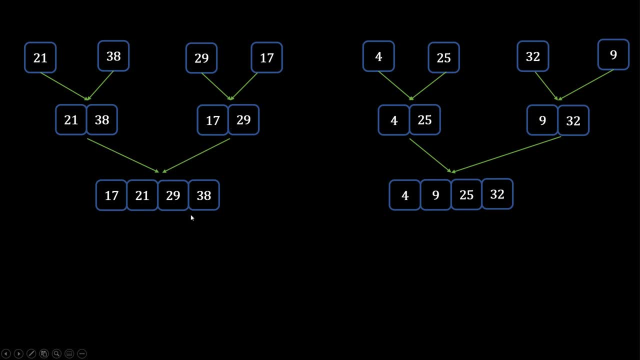 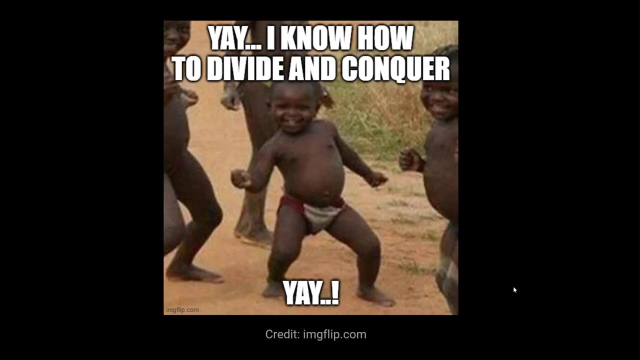 so you can merge them using the technique that we learned- and it looks like this similar thing is happening here- and then you sort these two as well into the array. so now you realize that by divide and conquer, we sorted our original array easily. yay, i know what is divide and conquer. yeah, bro. okay, the time complexity of this algorithm is. 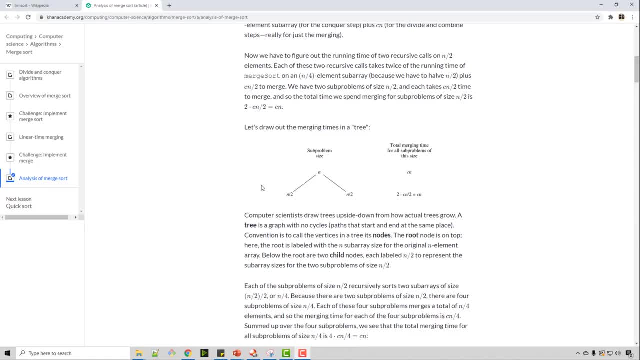 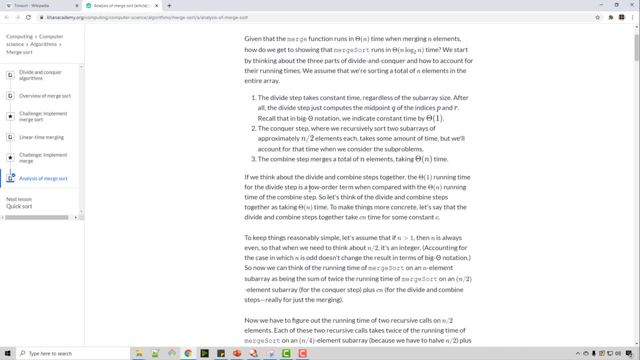 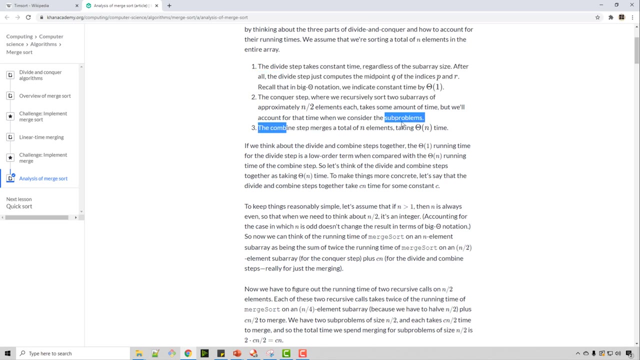 order of n log n. if you want to know how we arrived at that complexity, i suggest you read this article on khan academy. our original divide operation is order of one, because it's a constant time, then the combined step is order of n and then the actual merging and merging part uh is uh merging and sorting them is n log n total. 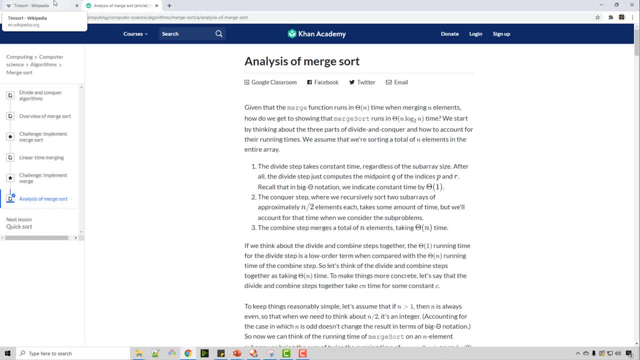 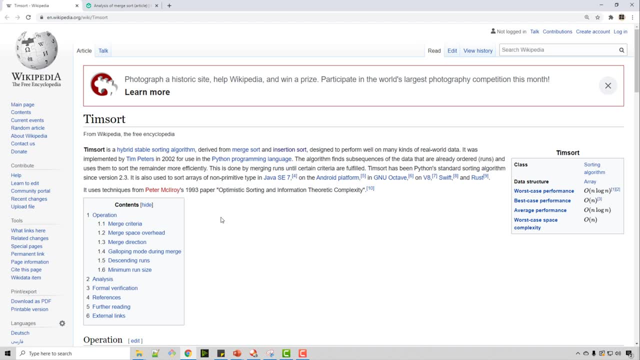 so just read through it, you will get an idea. now, merge sort is an important algorithm because it is used by python sort function. so when you call sort built-in function in python, it uses a technique called tim short, which is a hybrid algorithm that uses merge short and in. 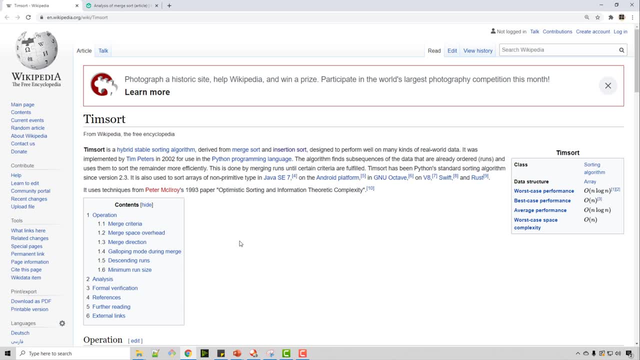 search and short. so you realize that mer shot is quite important. it gives you a very good time. complexity: we saw like things like bubble short takes order of n square, which is a lot of time, whereas match short takes only n log n, which is quite fast. let's go get into python coding now. 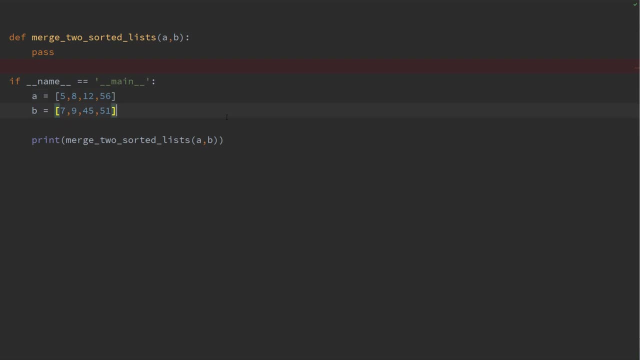 first thing i will do is write a code to merge two sorted arrays. so i have written this empty function and I'm passing two sorted arrays, so let's finish this function first, then we will write the code for merge short. so as we saw already that we are taking two, 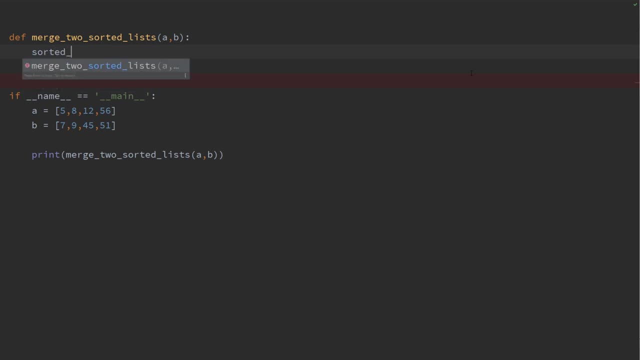 sorted arrays and creating a third array. so I'm just gonna call it sorted list and I will return that whenever that sorted list is prepared. so here we will be writing that code, the need. the thing you need to do is first get the length of both the list, A and B, okay, and then you will iterate through both the list. 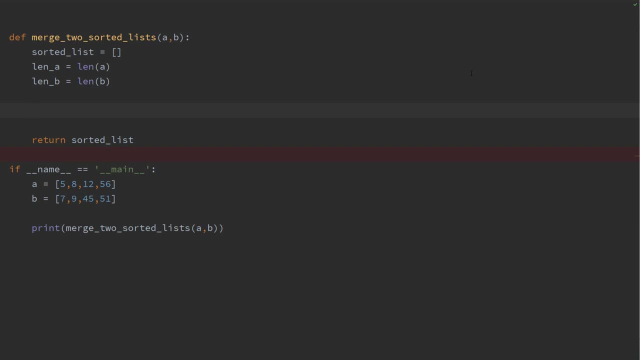 until you reach end of either of them. so you will say: while I is length, you know, and we just have to point out, let us, I is equal to J is equal to 0, and you will say: length of B. you're doing this because you want to stop. 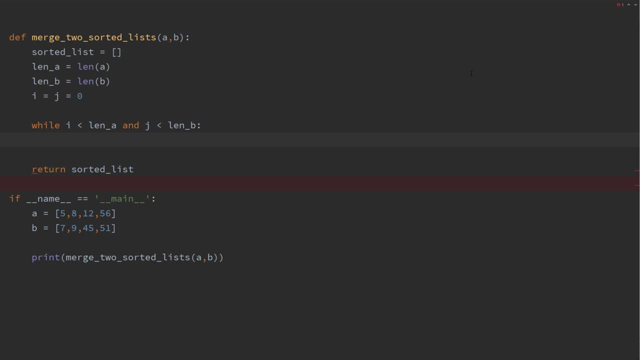 whenever you reach the end of either of the list now you first check the, you compare the element from both the list, right? so you say, if A of I is less than equal to B of J, which is in the second list, you have a element which is higher than the first list. so now you will put this particular element. 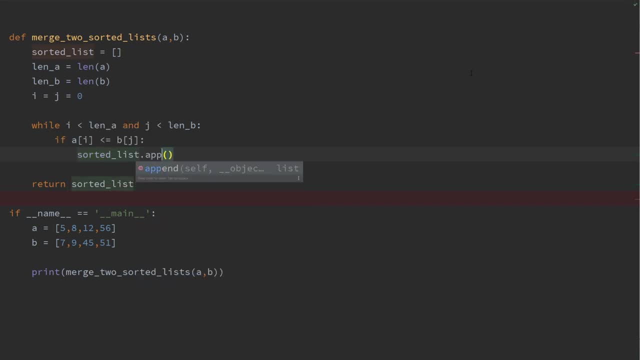 in a sorted list. so you will say sorted list, dot, append and append. you put A of I and then you of course increment I right, because you are inserting element to sort a list from A. that's why you are only incrementing I. you are not incrementing J, because your J pointer is still static. if you look at our 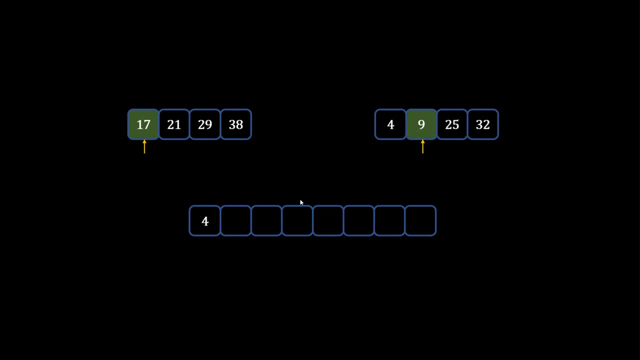 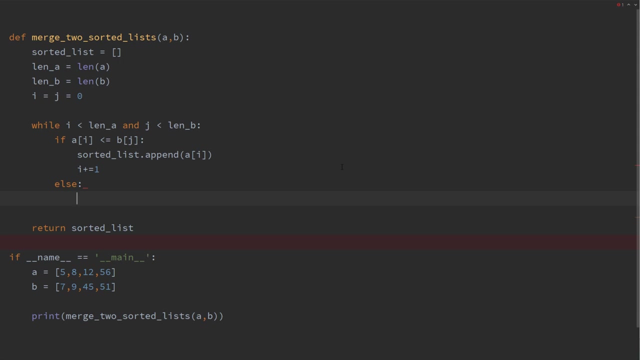 presentation. you see, if you are inserting 9 from the second list, you are not touching your pointer from the first list. so whichever list you insert the element from, you only move the pointer of that. so right now, this is I, this is J in the. else you find that the element in the other list is less than this. first, 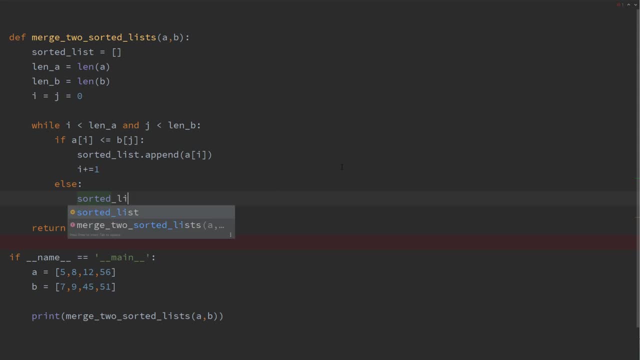 list. so you will now put that element in your sort list. so you will say: append B of J. guess what you need to do here? well, you need to increment J, all right. so I think the logic is kind of done. we iterated through both the list. 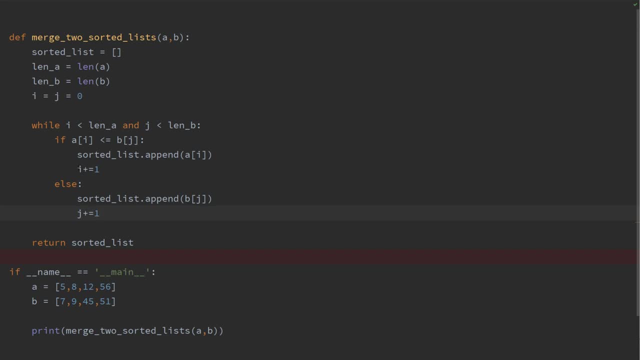 so I think the logic is kind of done. we iterated through both the list, so I, and from each of the lists we are maintaining the pointers, which is God- and you compare the element one by one and whichever element is less, you put it into sorted list and you return that. so let's execute and see what happens. 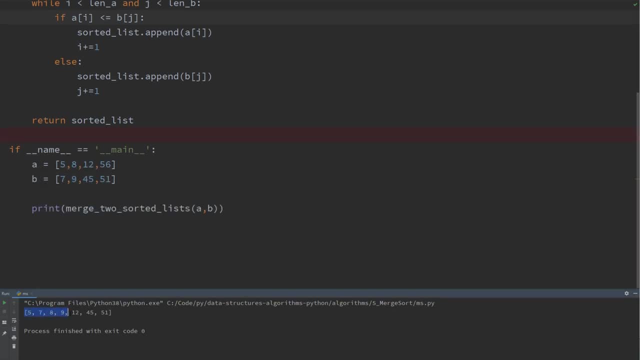 okay, so looks like it worked. five, seven, eight, nine, twelve, forty five, fifty- oh, I see fifty, six missing. any guess on why this happened? well, I think what happened was we reached the end here. okay, so let's say this condition: so we reach the end, and when you reach the end, just because you have end condition, this for loop will exit. 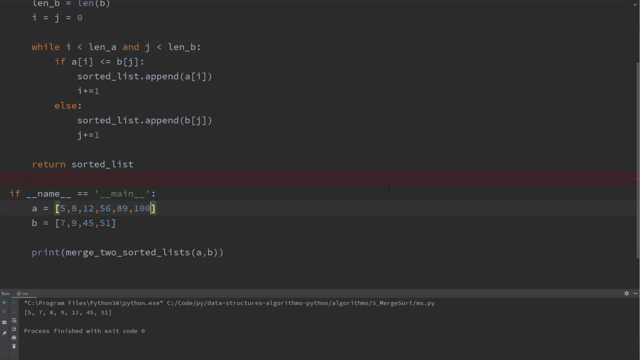 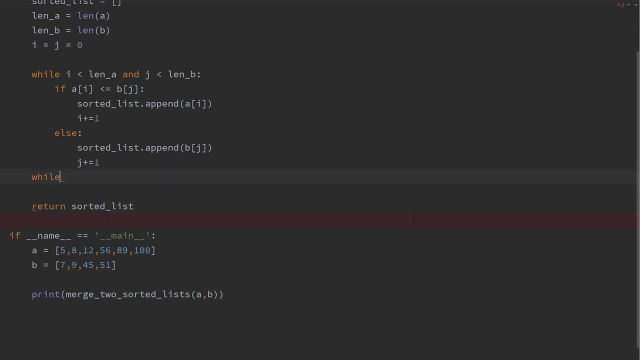 you can also have scenarios like this and see you will now miss all those elements. after this for loop exits, you will miss all these three elements, so we need to run one time loop on both the list actually. so what that loop will do is so you will say, okay, after i have exited this loop, which means 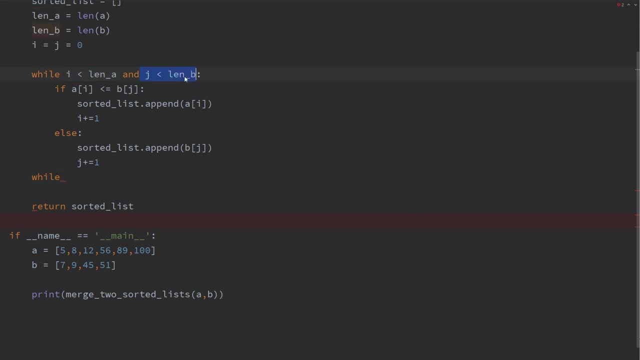 either this was true or this was true. if this is true, then i need to iterate to rest of the elements from this list and just directly append them. i will say i is list, then length of a sorted list, dot. append a of i and then i'm incrementing my i and you want to run the same loop for the another list, which is: 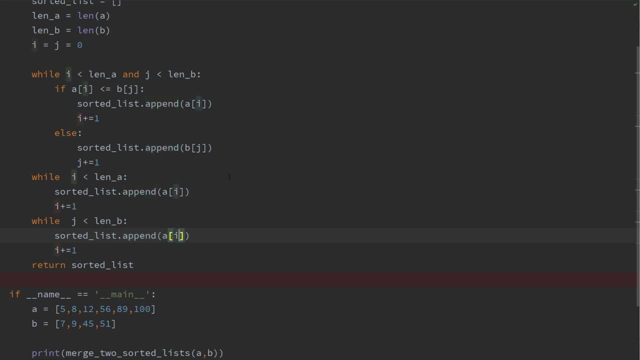 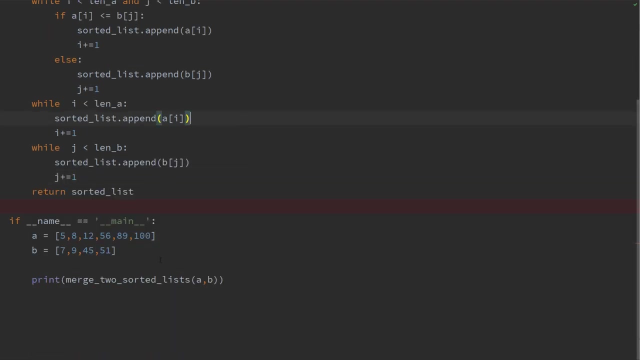 your b. so here you will say b. this is b of j, of course, and here you are incrementing j. i hope you're getting the point. if you don't just put a breakpoint in your pycharm and run it, i'm using pycharm zen mode. that's why you don't see any distraction here. 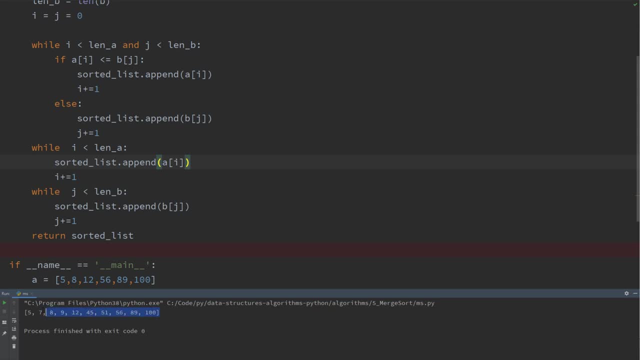 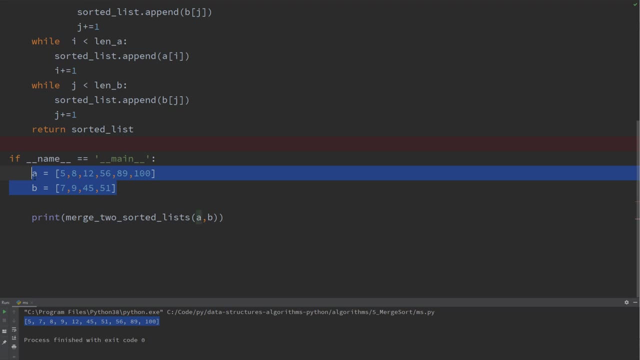 all right, so we have the function ready which can merge two sorted list. now we need to give our real list. so i'll remove this and i will give an unsorted array for shorting and i will probably write a function called merge short. okay, so i need to implement that. 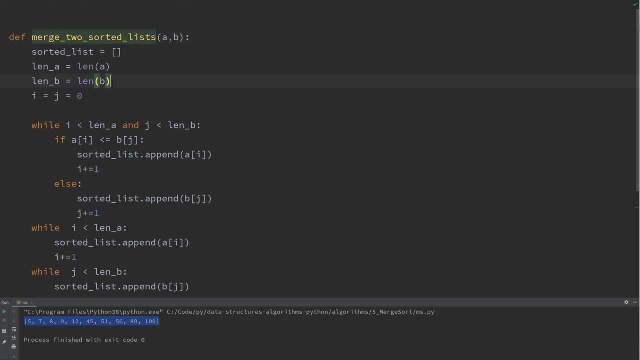 function, the utility function that we needed to merge two sorted arrays. we already have that, so now we are writing merge short function and okay, let's, let's think about it- what we need to write here. so this will be a recursive function, as you already saw in the presentation and for any 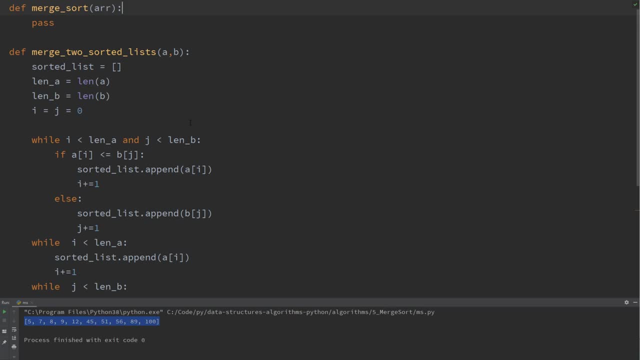 recursive function, you need to first take care of the exit condition. the exit condition was: whenever we have array of size one, you want to exit correct. so you will say: if length of array is less than equal to one, let's say it is one or zero, it's an empty list. 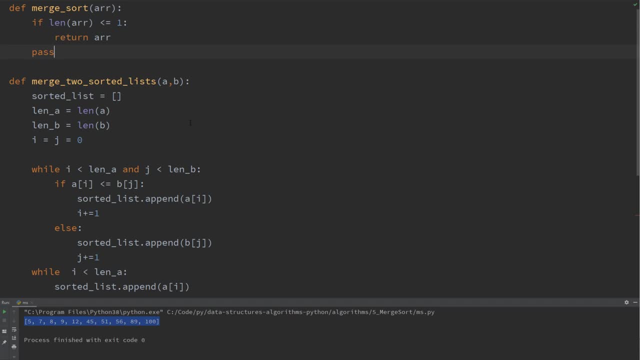 then you want to return that list. so this merge short function is returning the new sorted list, and if that is not the case, then you find the mid element, because you divide the array into two parts, left and right- and in python this is super easy once you have the middle. 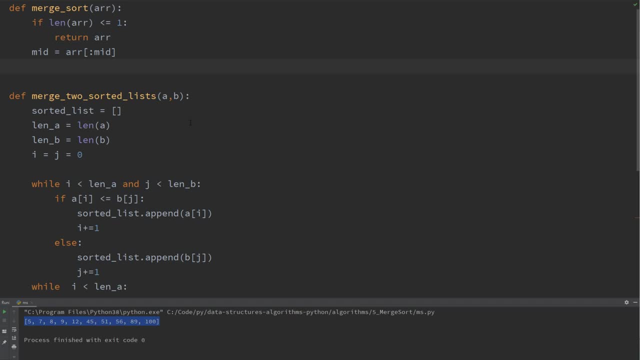 element. you can use the indexing. if you don't know about indexing and python basics, follow my python basic tutorials. you get an idea and you get left and right. right is elements starting from mid all the way till end. if you don't specify anything here, it means it sent. if you say six, 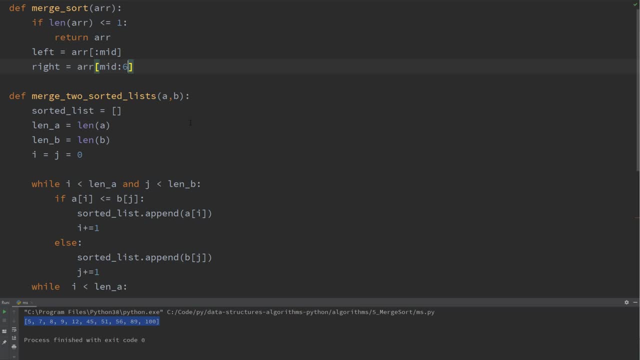 it is gonna be going till five. okay, now what i will do is see, i need to call. you know we need to call merge short function on both the left and right array. this is how you call it in a recursive manner, and once you can call merge short on left, you get a. 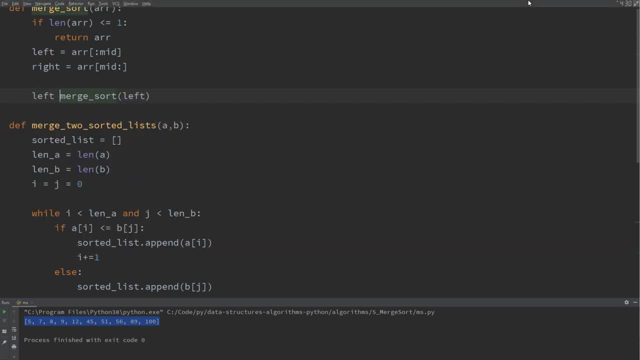 shorted left array. so I will store it in left and I will say: right is equal to merge short right. and once you get left and right, both are sorted. then of course you call merge to shorter list. so left and right, and you return that because merge short, by default it returns a. 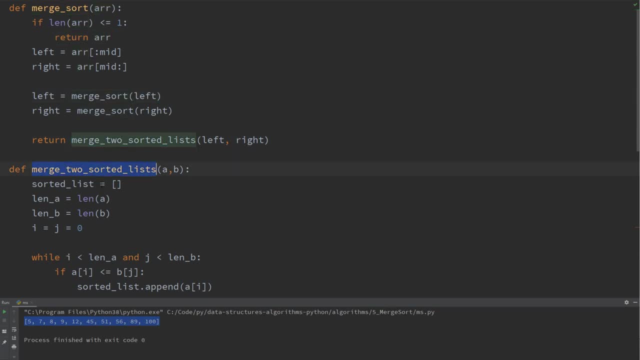 sorted array. so once you have sorted array- let's say two sorted array- when you merge this guy is also returning it. hence you need to return this as well. let's try it out. okay, mid is not defined. let's see. okay, so mid is nothing but the length of an 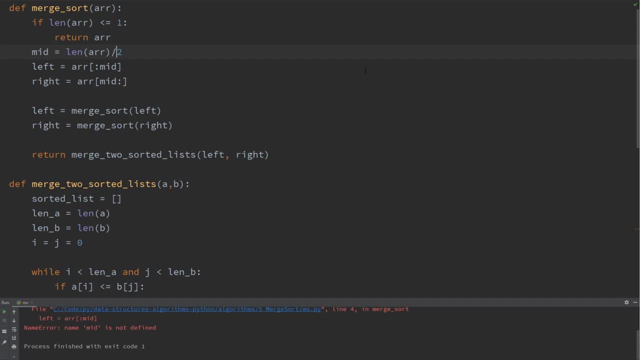 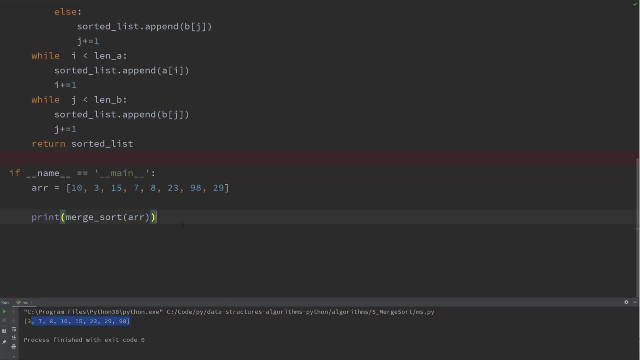 array divided by two. now, if you just do one divide, it will give you floating number. so if you do this, it will give you the integer number. see, my list is sorted. now you can see 3, 7, 10, 15. yep, so this worked, although this. 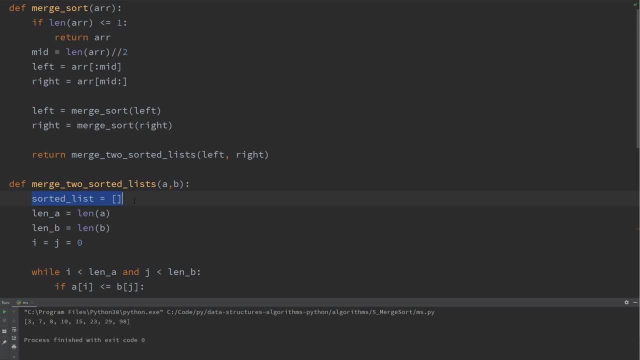 worked. this required creating new arrays all the time. you see you are creating new array, then you return it, so it's not optimal in terms of space complexity. so what if you can do everything in line in your original array itself? well then, that might be an efficient version of. 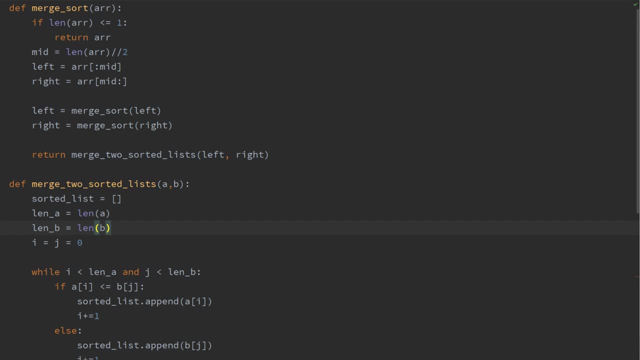 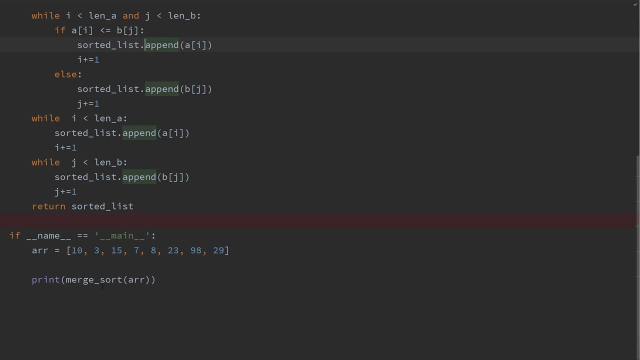 the merge short, so let's do that. so in that, what we are planning to do is basically something like: I don't have to return anything. see, if I do this and if I print array, it should be sorted. so you're sorting array in line. so for doing that we need to stop. 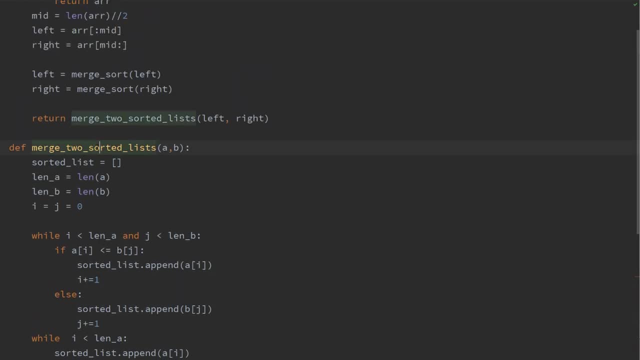 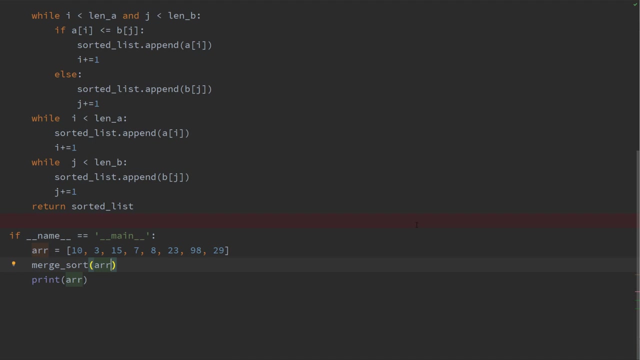 returning things first of all. so here I am returning. these two are shorted list. so instead of creating a new list, I let me remove that. what if I pass the original list here? so see, I have passed original list in my array, so let's start with merge short function first. so here in merge short. 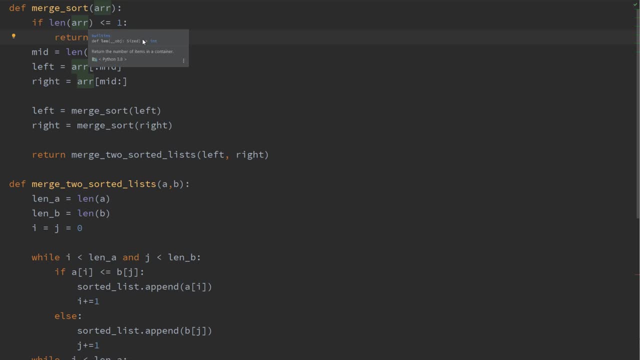 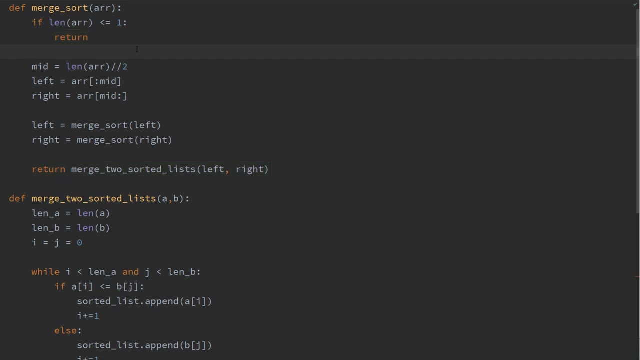 first of all, if the size of array is one, I don't want to do anything. it is already sorted, so let's not do anything. and then, here also, let's remove this, because when you call the merge short function, it is shorting this left and right array in line, and once you have these two arrays, you can just merge them. 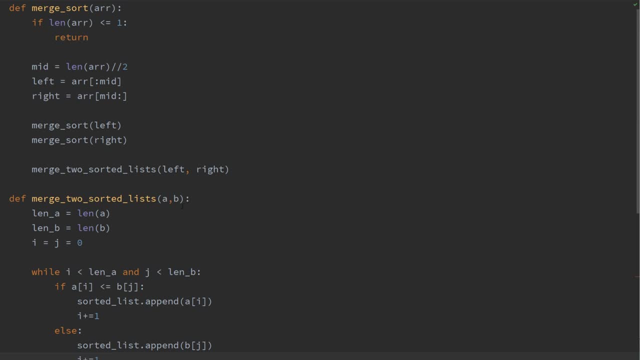 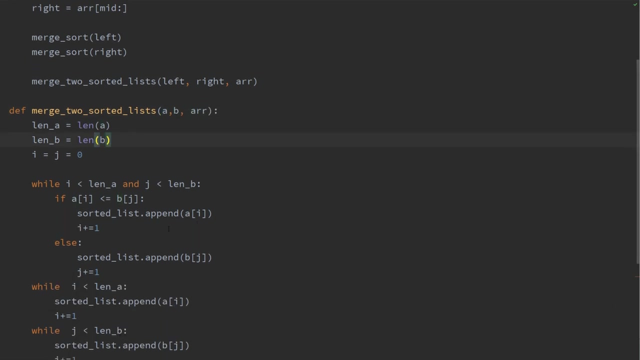 so now let's come to merge to sorted list. here I will pass an array because I don't have sorted list and I need some place to put my shorted elements, so I will do array here and then, hmm see, here I was putting, appending them to the sorted. 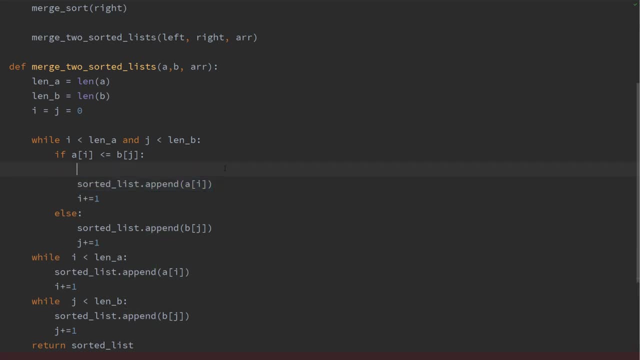 list, so that appending thing is gone. so here maybe I need to create a new index called K. this is the index into the sorted array, which is a RR here. so instead of appending it to a shorter list, what you can do is you can say: array of K is equal to a of I. so I'm just 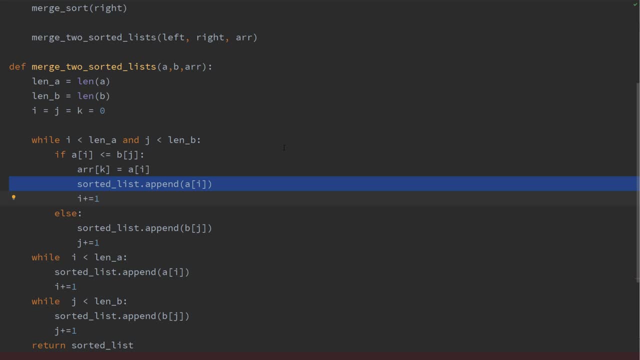 replacing this line. this line require me to create a new list. I don't want to create a new list to save my space, so I'm just using the original array, and here I will do the same thing, where I will assign B of J to something what is? 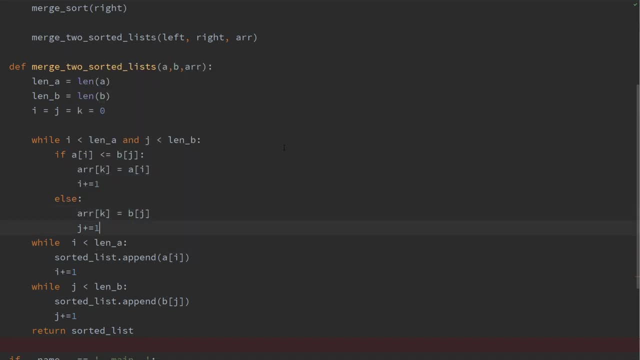 that array of K. okay, and in both the cases you to increment a because you are your appending element to your final list all the time. okay, you will do similar thing here as well. so here you will do assignment from array a and then increment a same thing here. 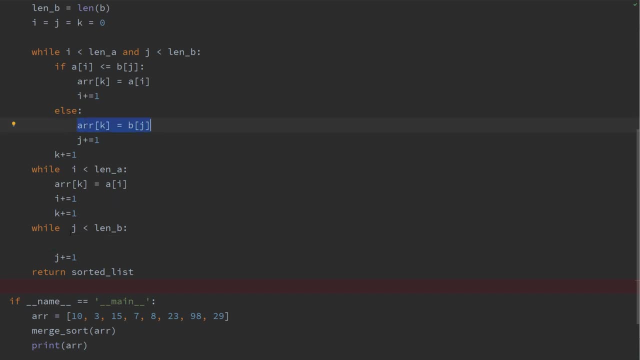 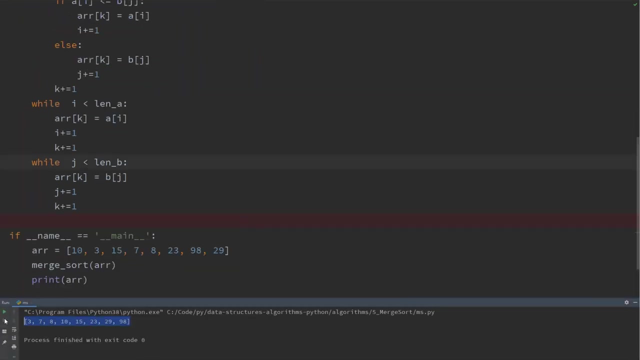 and increment k and you don't return anything because the inline array itself is shorted. okay, so it's the same code as previous one. i'm just optimizing my memory usage. right click, run and you see the array is shorted. now usually you want to run couple of test cases. 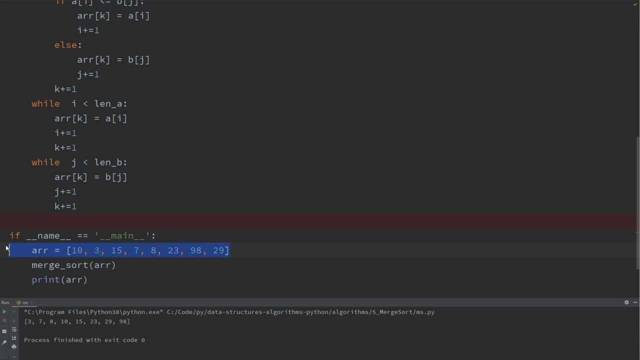 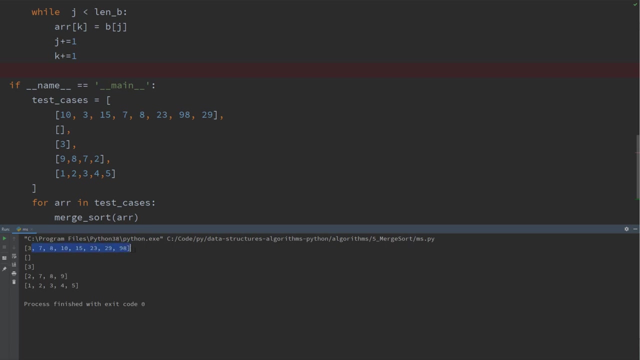 to make sure it is working for all the edge cases and so on. so i always have this habit of writing different test cases and i will do for array in test cases. so it will take one array, one by one, and then it will print it. wow, so that worked. you see. check each of this list. they are all sorted. i tried empty list. 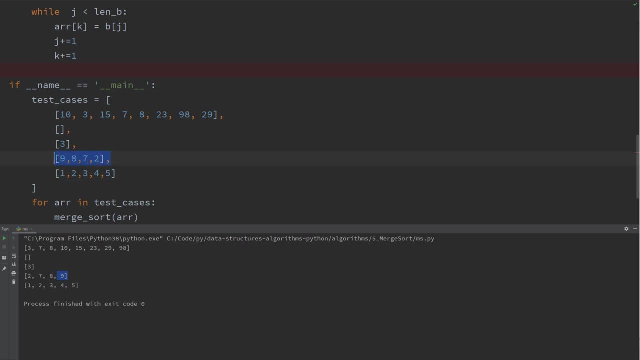 list with one element, uh list, that is reverse sorted list, that that is already shorted in a correct order and a random list, and it is passing all the test cases. so, hooray, good job, our merge short program is done. now let's move on to an exercise. 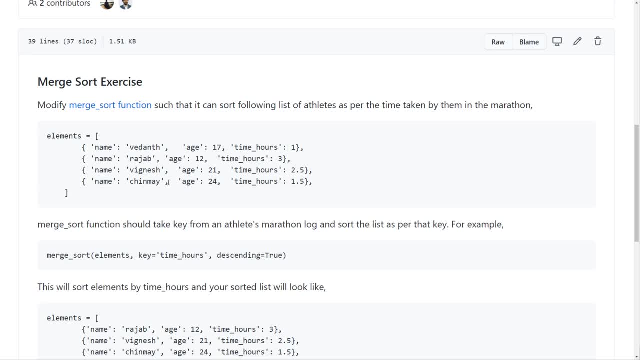 i'm gonna provide a link of this exercise in the video description below, so make sure you check the video description for the link of this exercise, as well as the code we covered in the video. what you have to do is you have list of elements which are like json objects.